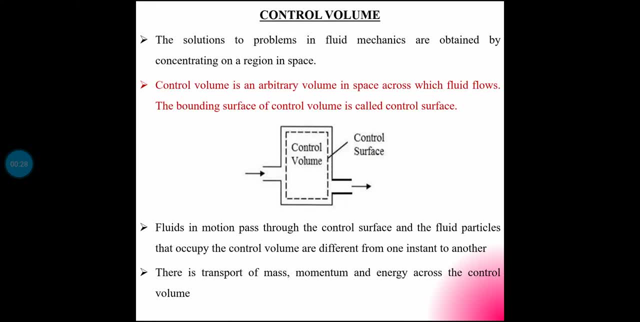 First topic, control volume. The solution to problems in fluid mechanics are obtained by concentrating on a region in space. Control volume is an arbitrary volume in space across which fluid flows. The bounding surface of control volume is called control surface. In fluid mechanics, control volume analysis is analyzed. 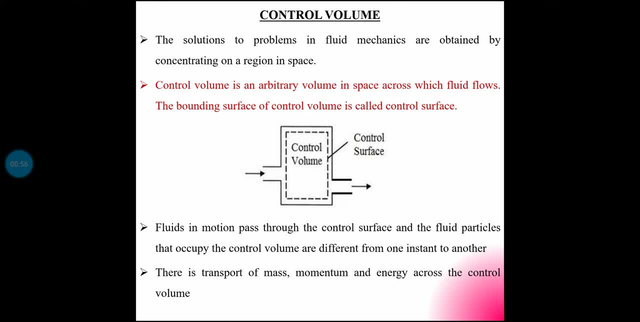 In another analysis. control volume analysis is analyzed In flow mechanics. control volume analysis is då the solution for fixed mass and finns possible acrossppings of closed system analysis. In closed system analysis the usable mass does not change. The mass normalizes, and aluntobecause of the limited enough space between the upper and lower boundaries, and in that lower boundaries, 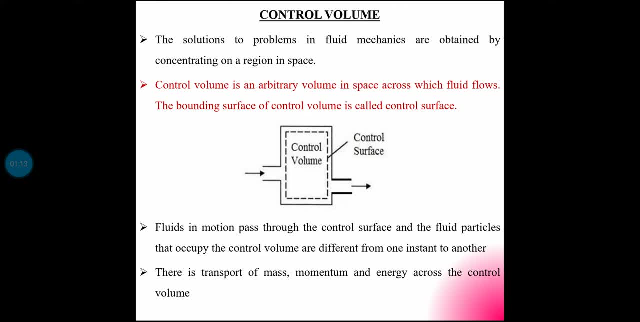 In flow mechanics the influence in naturally and Periods are died down to Lifezar. QSTA analysis is mostly the analysis of fluid volumes. QSTA analysis is another analysis of the count đầu volume of a fluid. QSTA is another analysis on the floor of the air. 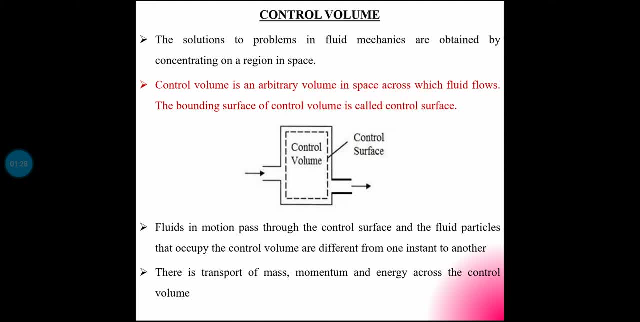 What is a volume? It is an arbitrary volume in space. The fixed volume that we choose is called control volume. It can be any shape. What happens inside that volume? Fluid enters and fluid leaves. That is, the mass of the control volume is not fixed. 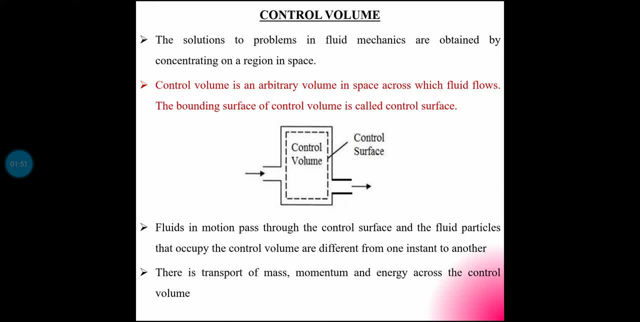 It changes Because fluid enters and fluid leaves. That control volume is considered as the bounding surface of the control volume. When it is a volume, there will be a surface that is bounding to it. What is the surface it refers to? It is a control surface. 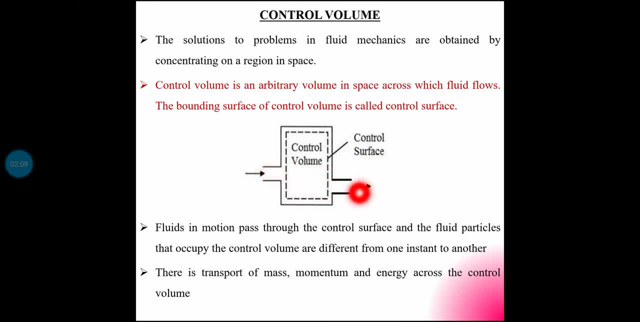 If this is my control volume, then fluid enters and fluid leaves, Otherwise the mass inside it is not fixed. If the mass is fixed, it is called a closed system. The mass enters and the mass leaves. This is called an open system or control volume. 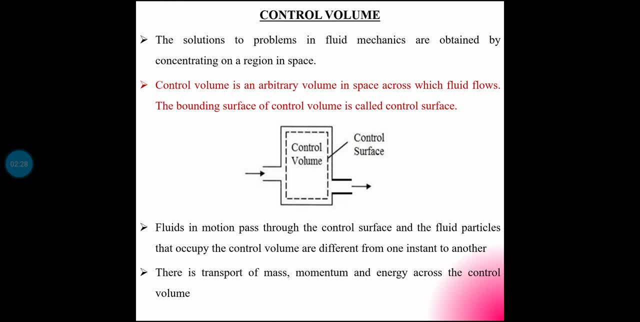 Fluids in motion pass through the control surface, And the fluid particles that occupy the control volume are different from one instant to another. There is transport of mass momentum and energy across the control volume. Here, at a time, fluid particles will be occupied. 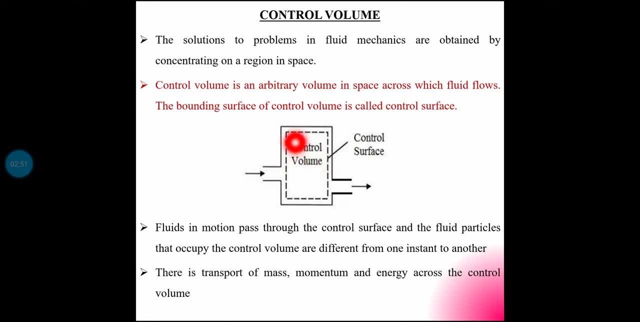 That same fluid particle will be there. It will be there in another instant. That means initially there will be a fluid particle. As time passes, the fluid particle will flow. At that time other fluid particles will enter into it. That is, the fluid particles that occupy here will be different depending on the time change. 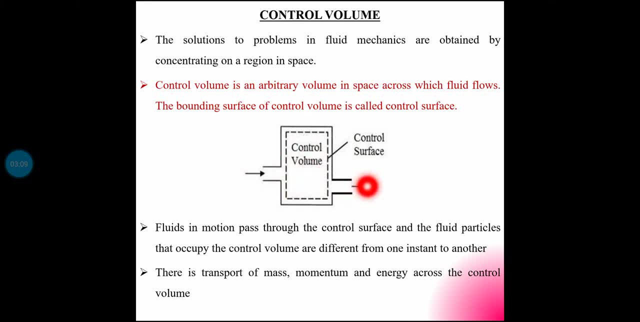 What does that mean? There is flow. The fluid enters and the fluid leaves. Otherwise, when the fluid enters and leaves, there is transport of mass momentum and energy across the control volume. The fluid particles enter and leave in the control volume. 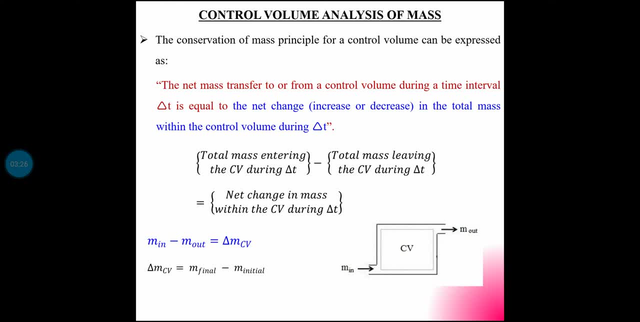 That is what I said. Next is the control volume analysis of mass. Just here, the control volume analysis of mass, momentum and energy. Just the outline of it. It does not go into more depth than the most basic fundamental concept: The conservation of mass principle for a control volume can be expressed as: 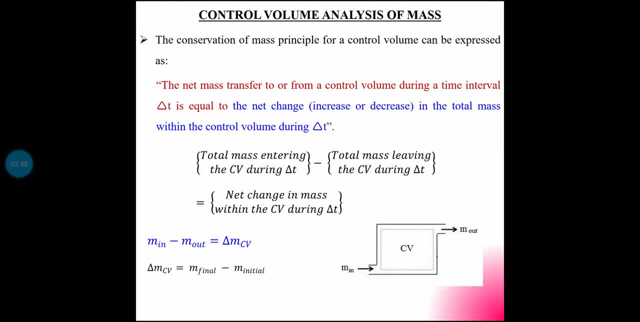 the net mass transfer to or from a control volume Or from a control volume During a time interval. delta t is equal to the net change in total mass within the control volume during delta t. What does the meaning of net mass transfer mean? Net mass transfer means mass in minus mass out. 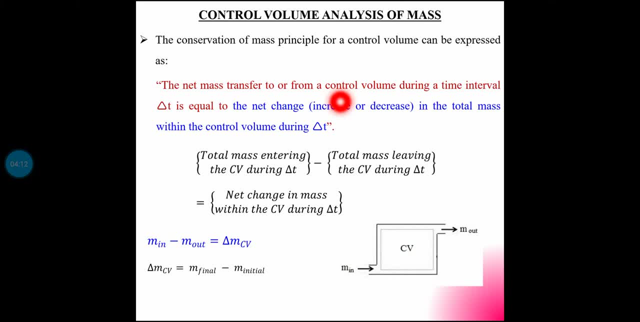 That is what net transfer means. Since mass enters, mass leaves, What is the difference between them? Net transfer, The net transfer during a time interval, delta t to the control volume. What does that mean? It is either increase or decrease. That is what net change means. 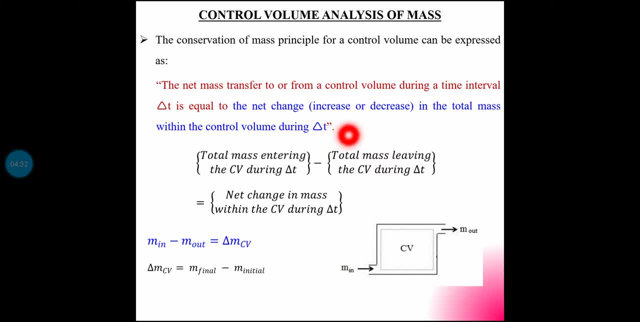 Net change in mass during the time interval delta t. What is the equation formula for that? Total mass entering the control volume during delta t minus total mass leaving the control volume during delta t is equal to net change in mass within the control volume during delta t. 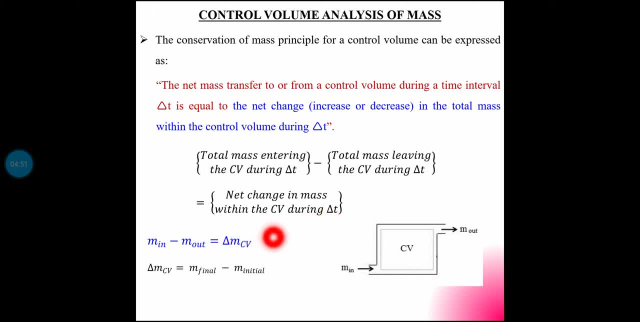 That is, mass in minus mass out is equal to delta m, cv. Here it is a unit kilogram. For example, the mass entering the control volume is 100 kg, The mass leaving the control volume is 50 kg. What is the net increase in mass during that time interval? delta t. 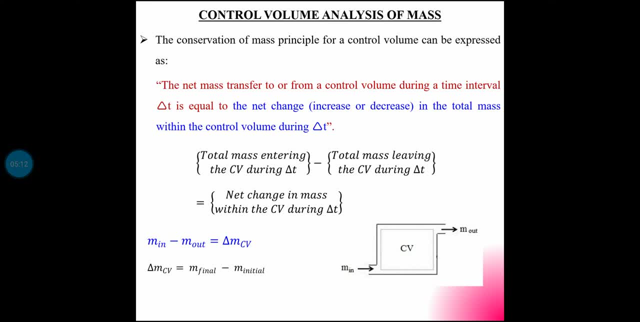 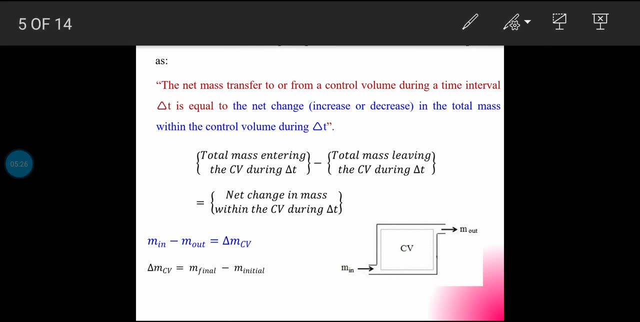 It is 50 kg, The rest is 50 kg. That is what the control volume analysis of mass or mass balance says. delta m, cv is the final mass minus initial mass. Let us see an example. I have taken a bath tube. 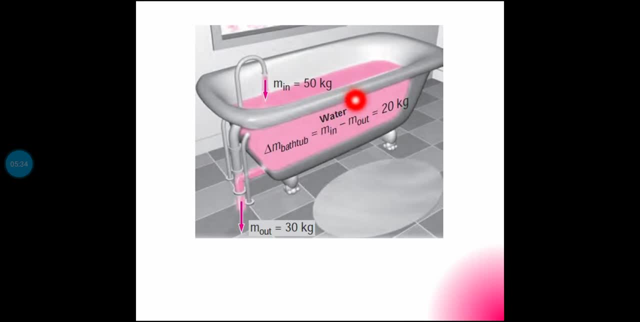 Initially, there is no liquid in it. Okay, the initial mass is 0.. What happened during a particular delta t time interval? 50 kg of mass entered into it. How much is left? in that same time interval, 30 kg is left. 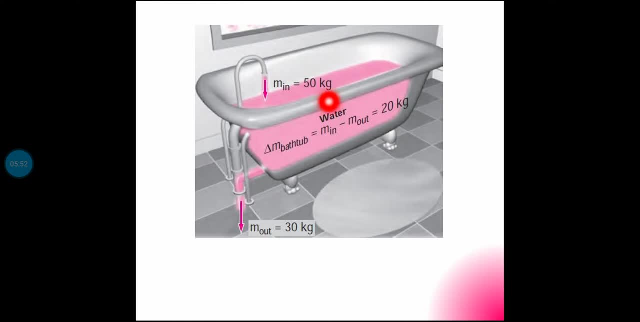 What is the rest? That 20 kg is the increase in the control volume. Okay, that is what the mass balance says. What is entering minus leaving? That is the net change. That is the increase in the mass of the control volume. 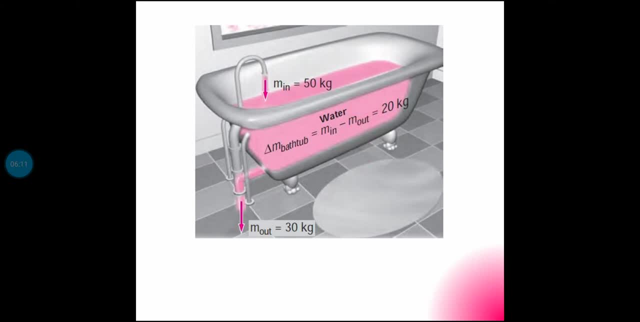 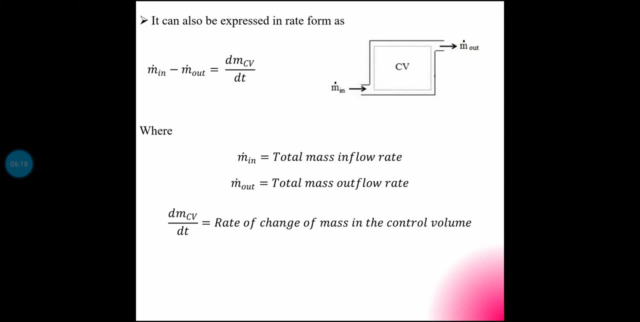 This is the mass balance. This is the mass balance. Now the unit is in kilograms. If we convert it into the rate form or the kilogram per second form, we get m dot in minus. m dot out is equal to d by dt of m cv. 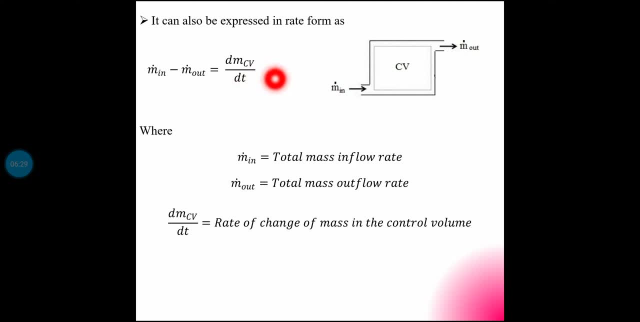 It is converted into the rate form. That means the unit is converted into the kilogram per second. What is m dot in Total mass inflow rate? Total mass inflow minus total mass outflow, This is equal to rate of change of mass in the control volume. 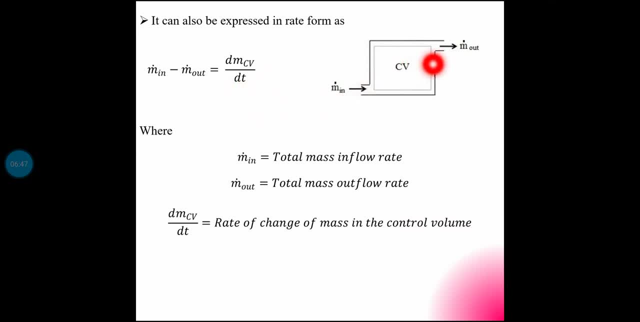 I am just writing the rate formula for this concept. Normally there would be only one inlet. Here I have shown only one inlet and one outlet. There would be one more inlet and one more outlet. That is what we call total mass. 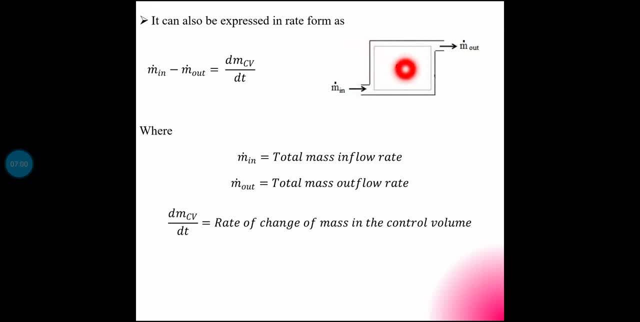 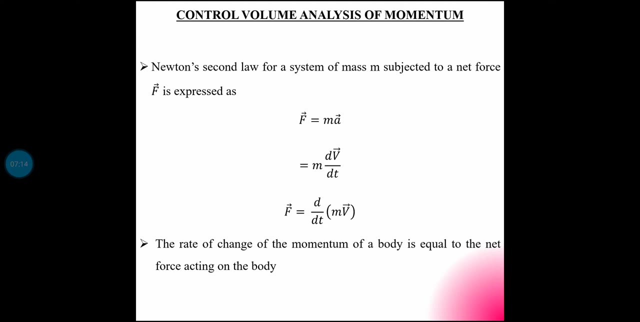 The entry through all the inlets and the outflow through all the outlets. This is the control volume analysis of mass. This is the most basic concept. Next is the control volume analysis of momentum. The most basic law in momentum analysis is Newton's second law. 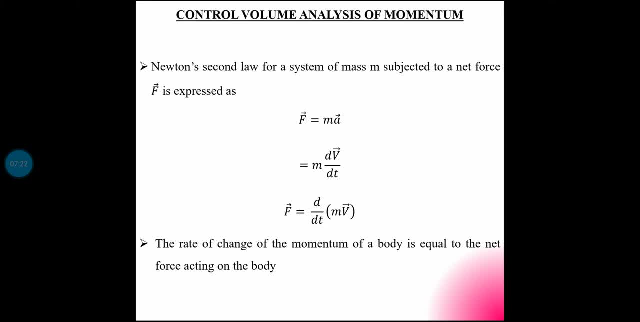 Newton's second law for a system of mass: m subjected to net force, F is expressed as: F is equal to m. I have written here the Newton's second law for a system of mass. This is a closed system. The mass is not changing. 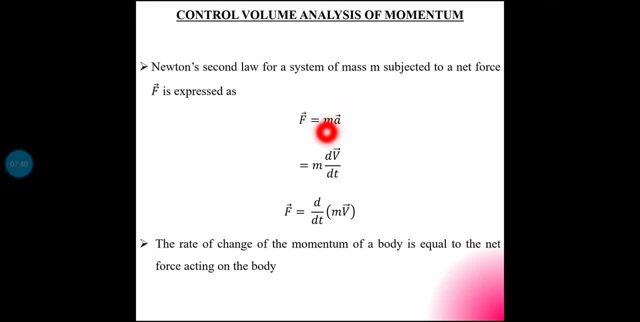 What is m? There is a system containing a mass called m. This is written for that. This is written for a closed system, not for a control volume. F is equal to m. Now how can we write acceleration dv by dt? 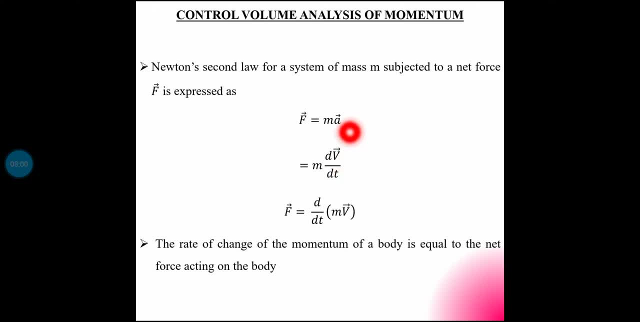 What is v? Velocity Acceleration is the rate of change of velocity. Then I have said that this is fixed mass, This is fixed mass. A is the acceleration. At that time, the force is F, The mass is fixed. 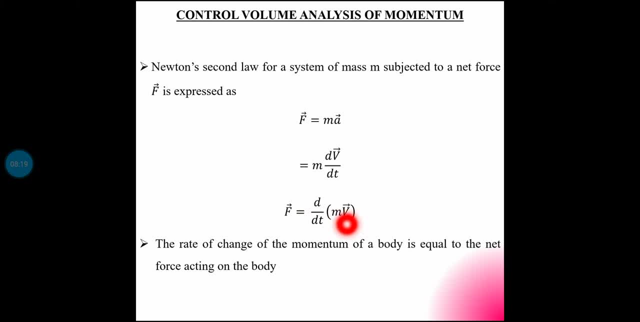 Take this into the differential d by dt of mv. What is the velocity of mass? It is momentum. F is equal to d by dt of mv. What is the statement formula? The rate of change of momentum of a body. This is the rate of change of momentum. 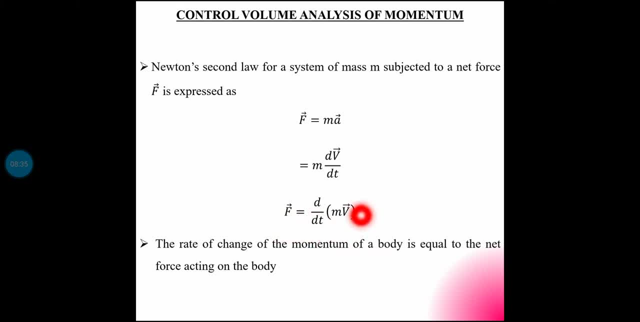 This is equal to net force acting on the body. The rate of change of momentum of a body is equal to net force acting on the body. Okay, Who is this for? It is for a controlled closed system. It is for a controlled mass. 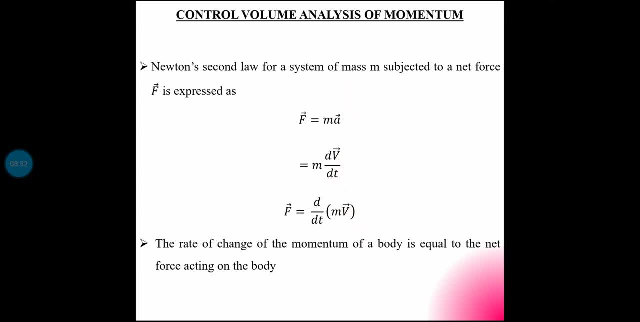 That is why it is written here. Normally, what we need here is a controlled volume. The basic law is the same, But there is a slight difference in the equation. The system approach is the closed system approach. There is a slight difference in the control volume analysis. 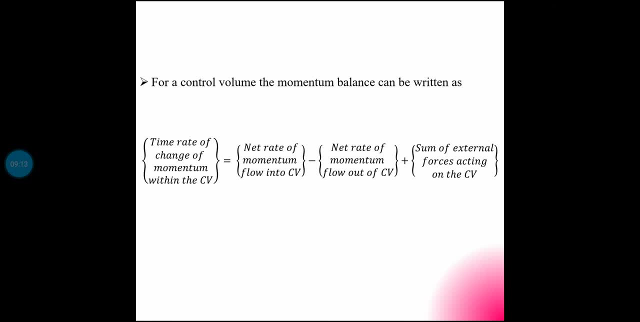 For a controlled volume. the momentum balance can be written as: Let's look at the case of a controlled volume. How will it change? The time rate of change of momentum within the controlled volume is equal to net rate of momentum flow into the controlled volume. 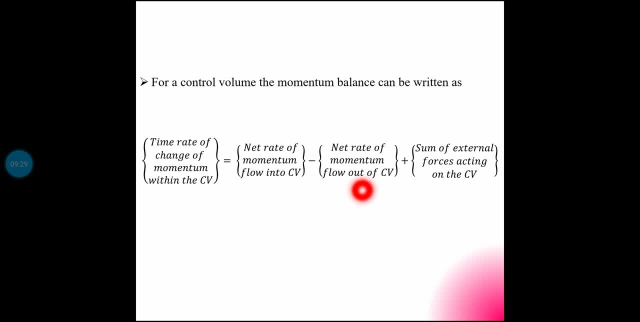 minus net rate of momentum flow out of the controlled volume, plus the sum of external forces acting on the body forces acting on the control volume. This is the momentum variance of the control volume. That is, the time rate of change of momentum within the control volume. 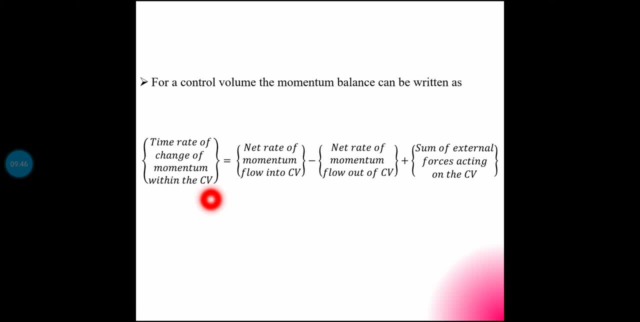 The change of momentum according to the time of the control volume. What is that? Net rate of momentum inflow minus net rate of momentum outflow? That is, the inflow minus outflow momentum of the control volume plus the net external force acting on it. 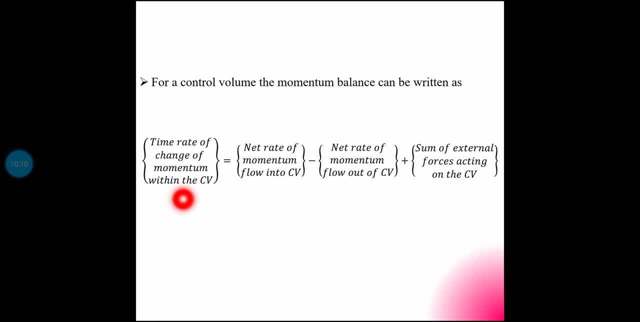 The sum of these two is the time rate of change of momentum of the control volume. The basic equation is: F is equal to d by dt of MVN. What is the difference between the control volume and the control volume? There is a mass flow. We can write that down. 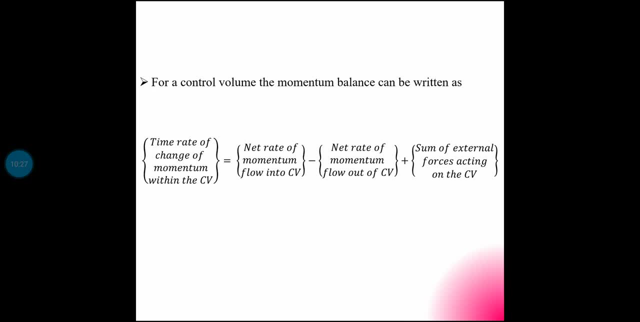 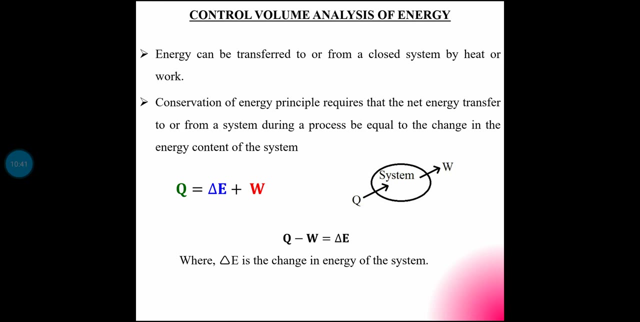 The system approach is related to the control volume approach. In fluid mechanics there is a theorem called Reynolds transport theorem. That is, the system approach is related to the control volume approach. Next is the control volume analysis of energy. Energy can be transferred to or from a closed system by heat or water. 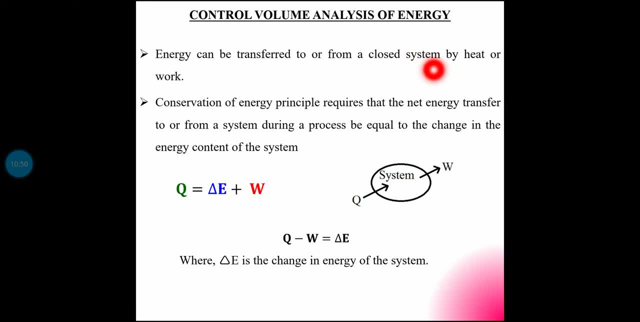 Where do I start? The closed system starts with fixed mass. After that we can go to the control volume analysis. This is fixed in a region. The most basic element of the energy analysis is the energy conservation principle. The energy can be transferred to or from a closed system by heat or water. 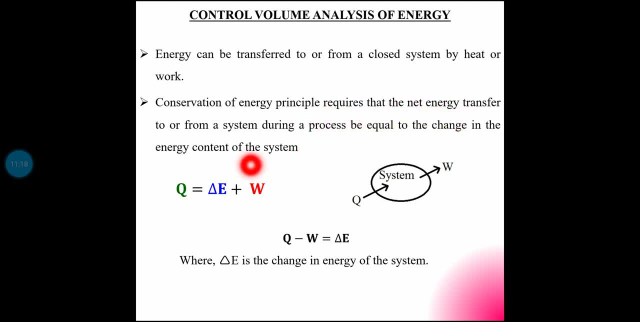 The conservation of energy principle requires that net energy transfer to or from a system during a process be equal to change in energy content of the system. What does that say? What does that mean? A system, a closed system, where the mass of the system does not change? 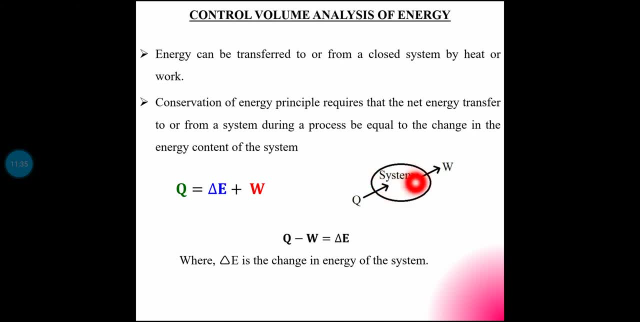 The mass does not enter or leave. The mass of the system is fixed. The energy transfer to that is either heat transfer or work transfer. Either heat transfer or work transfer. What is the energy conservation principle of that Net? energy transfer to or from the system during a process must be equal to change in energy content. 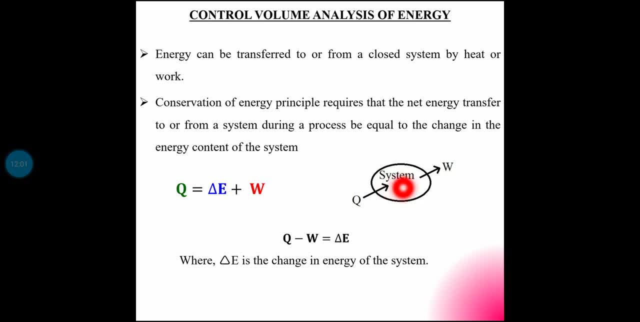 I am giving Q amount of heat to that system, It is doing W amount of work. The rest will be the energy changes in that system. That is what it is saying. Now I have given 100 kJ of energy. That is 70 kJ of work. 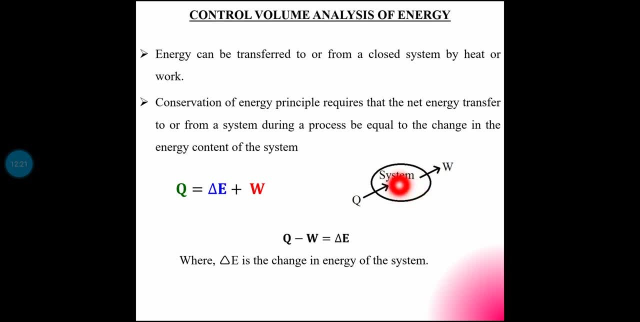 The remaining 30 kJ is stored in that system, Or the energy of the system increases. That is what the equation is saying. Q is equal to delta E plus W, Or the difference between Q and W, The energy given minus the energy left. 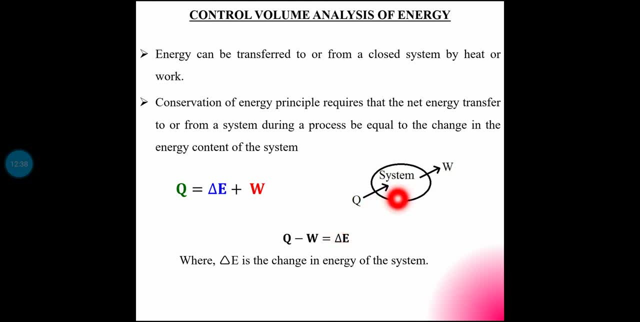 That is what the change in energy of the system becomes. The initial energy of the system will be there. After that, the rest will be added. That is what it is saying as the change in energy, Where delta E is the change in energy of the system. 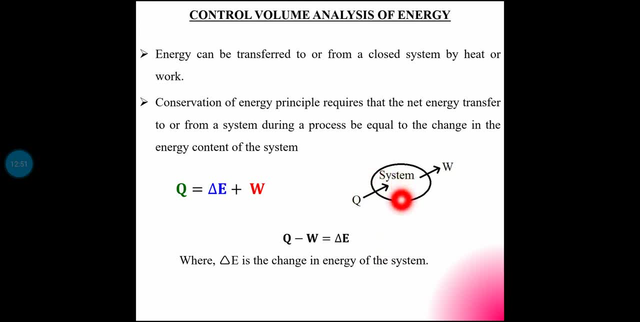 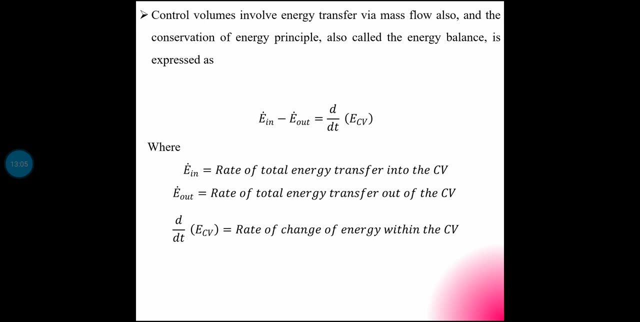 That is, Q minus W is equal to delta E. This is the energy balance of a closed system. Now what is the change in the control volume? There is mass in and mass out. There is no mass entry here. Now let's see how to write the control volume. 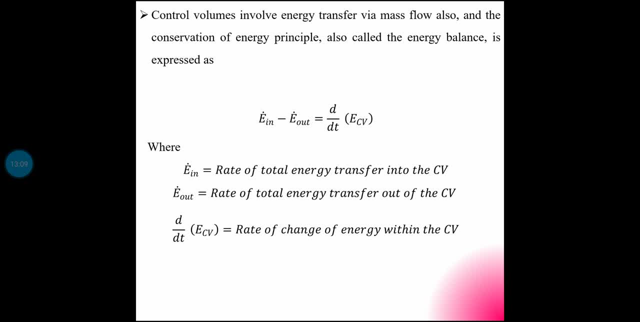 Control volume involves energy transfer via mass flow also, And the conservation of energy principle, also called energy balance, is expressed as: How does that change in terms of control volume? Let's see Energy in Rate of energy. in minus rate of energy, out is equal to d by dt of E cv. 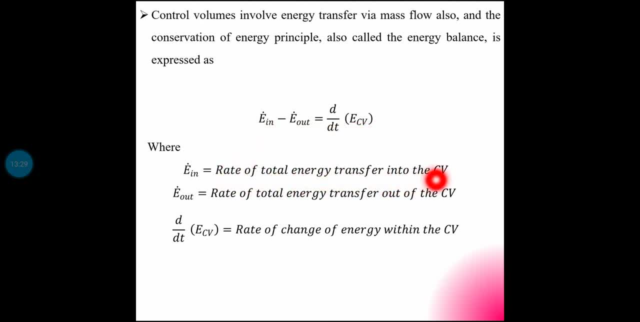 What is this? Rate of total energy transfer into the control volume minus rate of total energy transfer out of the control volume is equal to rate of change of energy within the control volume. I have already discussed the same concept of a closed system, But there is an additional flow here. 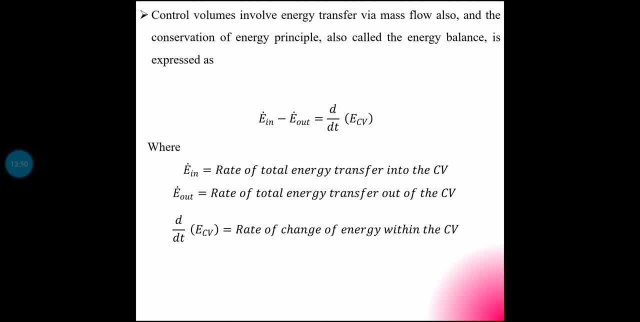 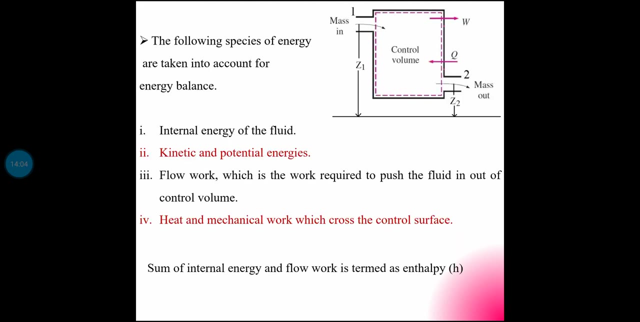 What is this? That is, rate of energy transfer into the control volume minus rate of energy transfer out of the control volume. What is this? Rate of change of energy within the control volume is equal to d by dt of E cv. I have shown a control volume here. 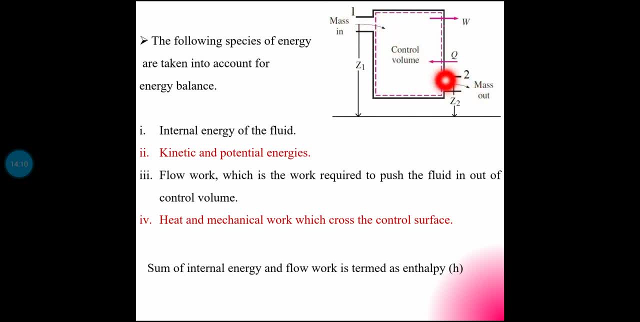 For that, I have shown only one inlet and one outlet. Normally there will be multiple inlets and multiple outlets. Just to write the equation, I have shown one inlet and one outlet. Just to write the equation, I have shown one inlet and one outlet. 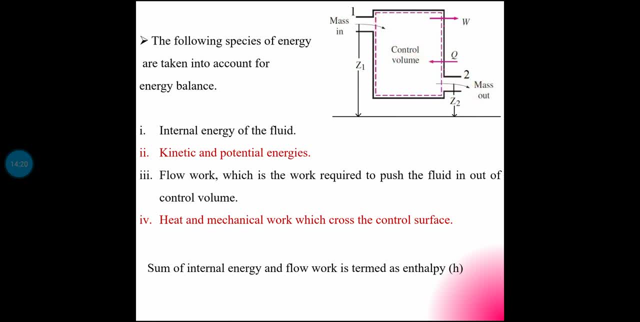 Just to write the equation, I have shown one inlet and one outlet. So how does the balance of energy exist? See the equation here. What are the energy species considered at this point here? The internal energy of the fluid. What are the kinetic and potential energies considered here? 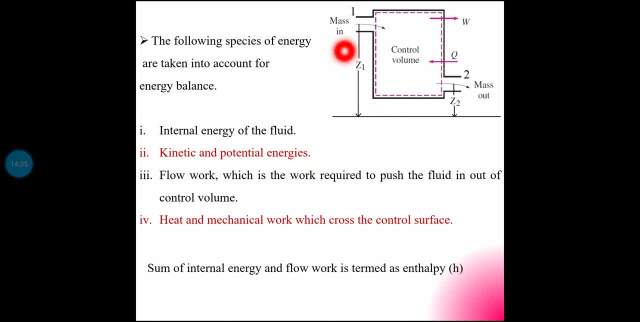 Flow work. The fluid is going to push the energy towards another. The fluid is going to push the energy towards another location. flow energy is actually the energy that the fluid possesses. that energy helps the fluid to shift from one location to another. that energy should be considered. 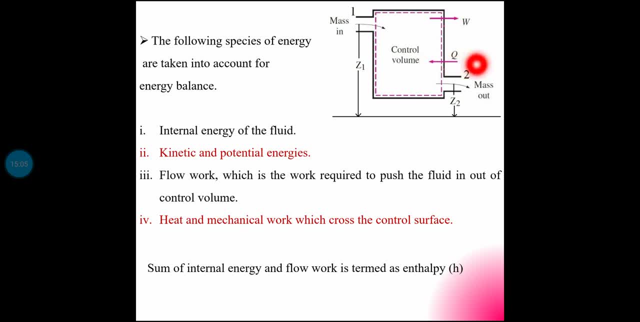 heat. there is a heat transfer into the control volume. heat will be in and heat will be out. it will be working on top of the control volume. control volume is considered as the device that normally takes control volume. it will be working on top of it. this control volume is a turbine. 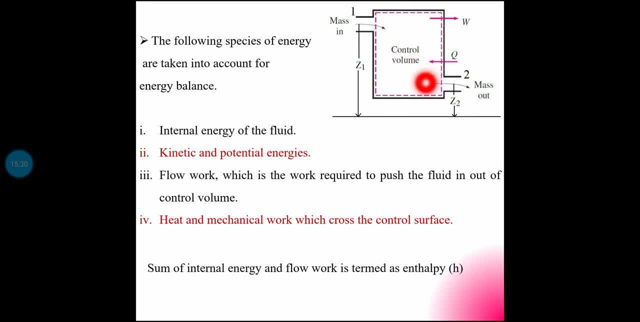 turbine is the control volume of a turbine. there will be heat input into it. there will be heat output due to heat and friction. it will be working on top of it. the turbine is a device that takes the work output. that is why it is marked here. control volume is generally mentioned. 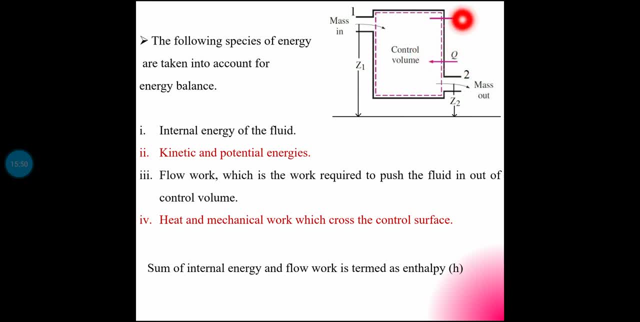 there will be heat transfer into it, or there will be heat transfer out of it, or there will be work transfer into it, or there will be work transfer out of it. what will happen? the energy that is considered here is internal energy, kinetic and potential energy flow work. 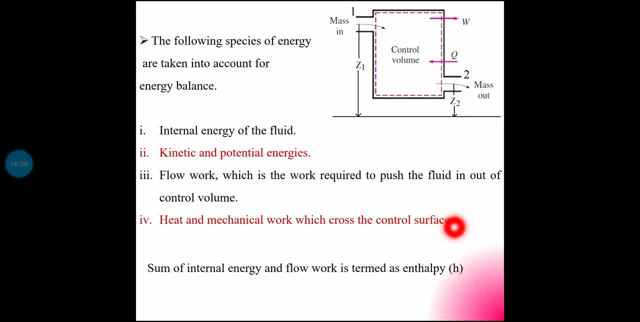 as well as heat and mechanical work which cross the control surface here, internal energy, flow work, internal energy- normally U represents flow work, PV. what is the sum of these two? have you already learnt sum of internal energy and flow work? for that Nthal P, H is denoted. 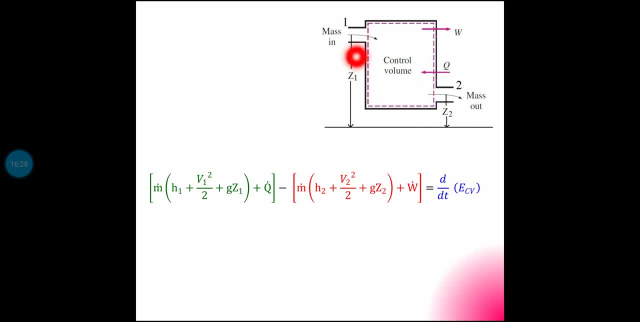 now, what is the energy balance of this? entering minus leaving? total rate of energy: entering minus total rate of energy leaving. what should be the difference? change in energy of the control volume: time rate of change in energy of the control volume. ok, according to this figure.